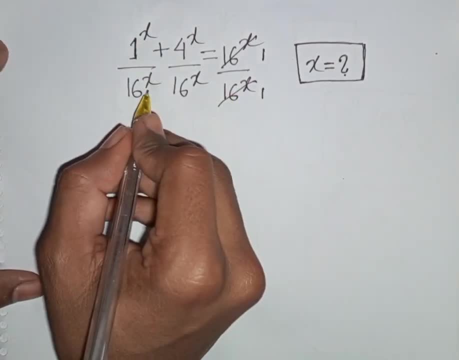 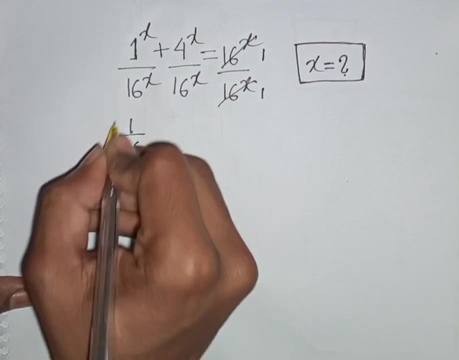 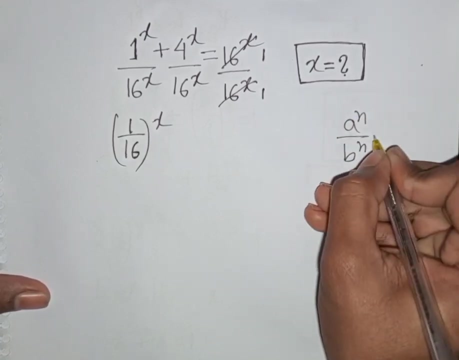 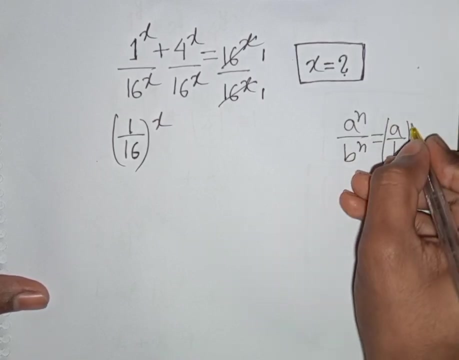 here: 1.. Now 1 power x divided by 16 power x, that means it will be 1 over 16. then bracket common power x. According to this formula: a power n over b. power n is equal to a over b. then bracket common power n. That means n, n. 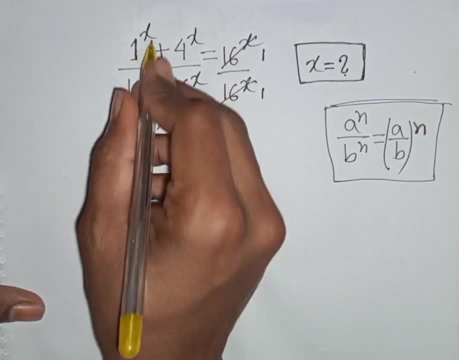 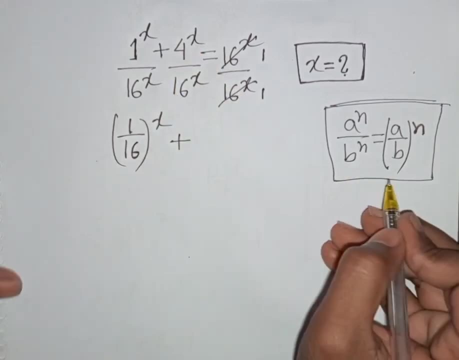 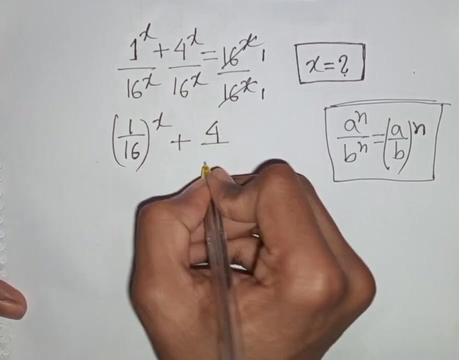 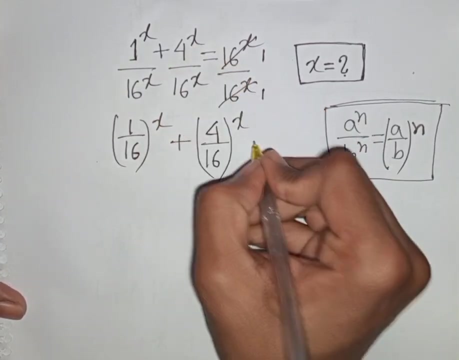 Same power but different base. Here x, x, same power but different base. Then plus again: x, x, same power, but different base. So according to this exponential rule you can write here: 4 over 16, then bracket common power: x is equal to 1 divided by 1.. That means it will be 1.. 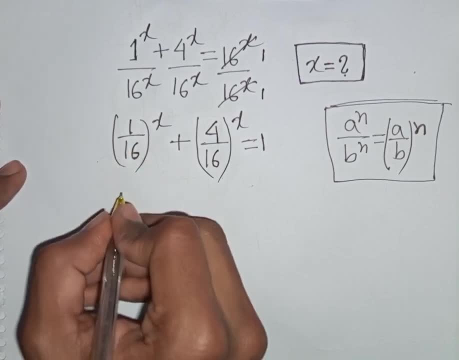 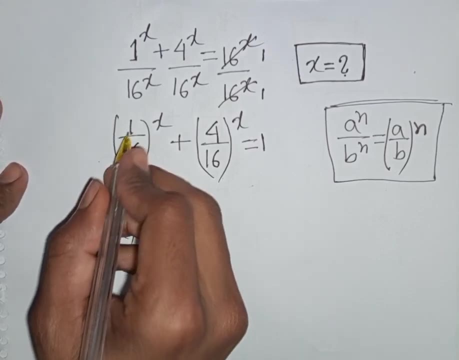 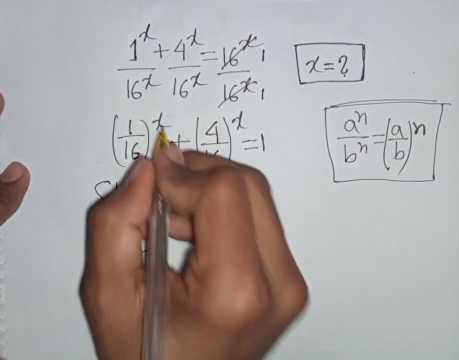 Now 1 by 16 can be written as 1 by 4 bracket: power 2. 1 square is same as 1 over over 4 square is same as 16.. Then this first bracket can be written as second bracket. then power of x plus we see 4. 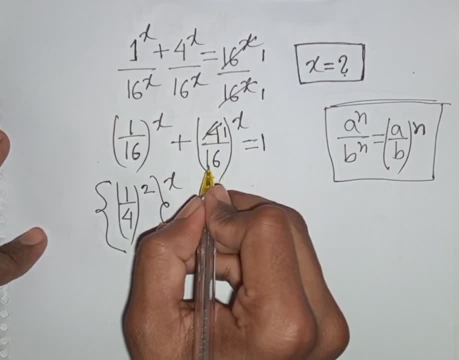 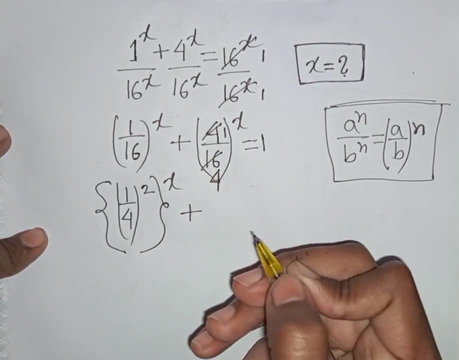 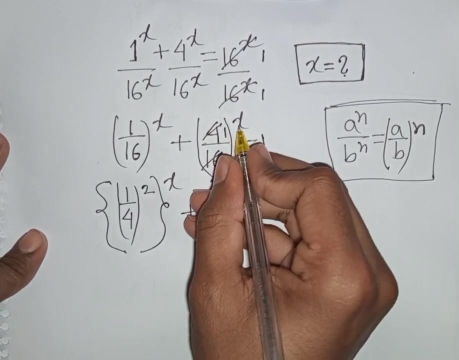 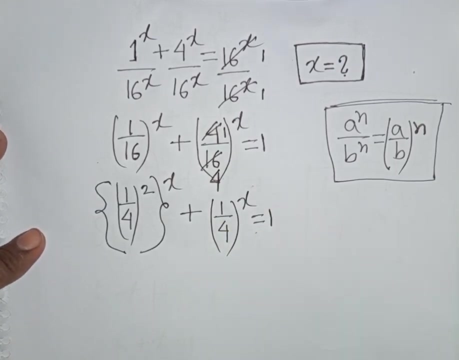 divided by 4, that means it will be 1.. 16 divided by 4, that means it will be 4.. So we have 1 over 4. then bracket power x is equal to 1.. Now Here you can apply this exponential rule. 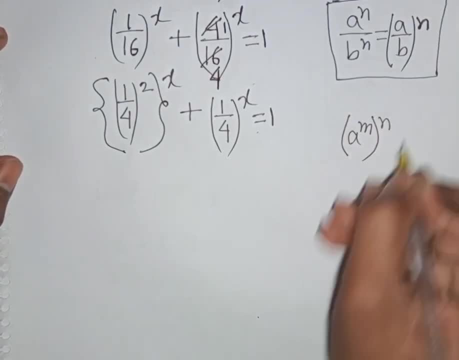 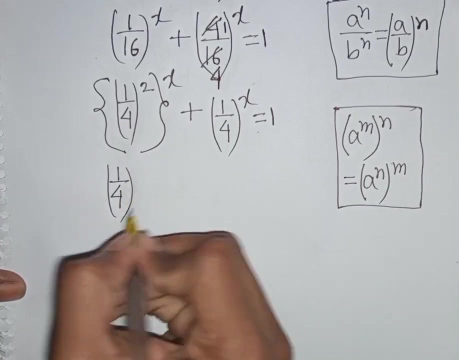 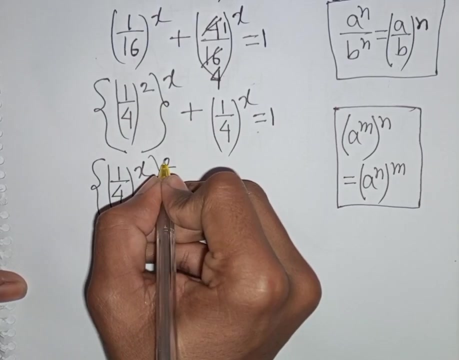 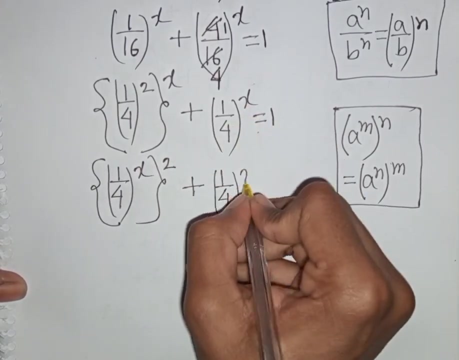 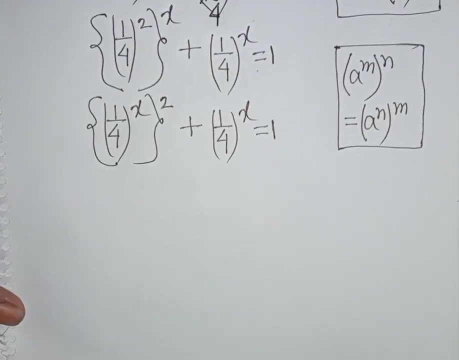 That a power m bracket power n is equal to a power n power M. So according to this rule I can write here: 1 by 4 bracket power X, then second bracket power of 2, then plus 1 by 4 bracket power X is equal to 1.. Now we see 1 by 4. 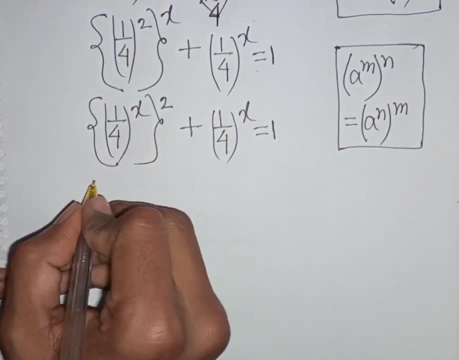 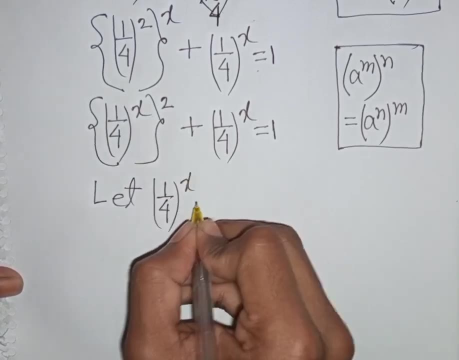 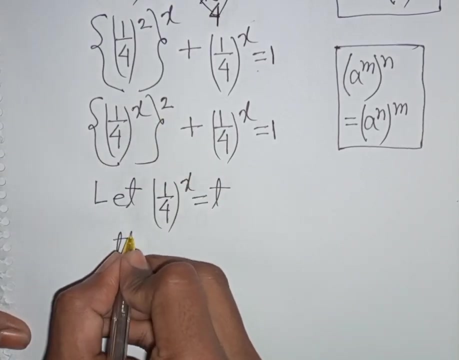 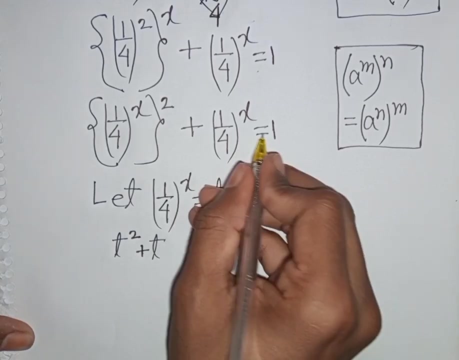 bracket power X: 1 by 4. bracket power X- both term is same, So let 1 by 4. bracket power X Is substituted by T, So our equation will be: T square plus T then is equal to 1.. Now 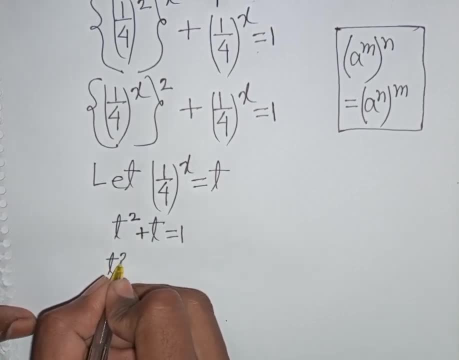 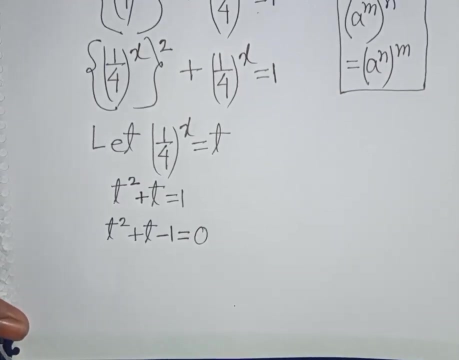 I can write here: T square plus T, then this plus 1, take to the left side, so this will be minus 1.. Okay, Okay, then a is equal to 0.. Now here I can apply quadratic formula. So you can write here: 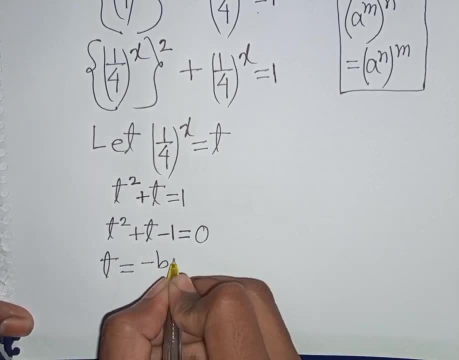 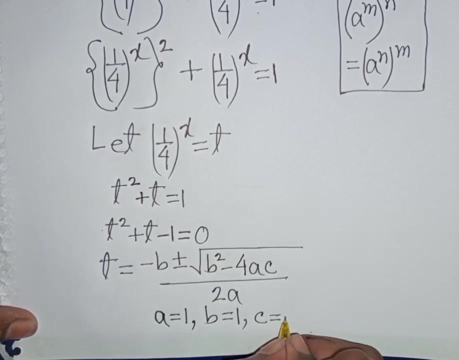 t is equal to minus b, plus or minus a. square root of b square minus 4ac divided by 2a. Here a is as 1, then b is as 1.. After that c is as minus 1.. Now we can write here t: 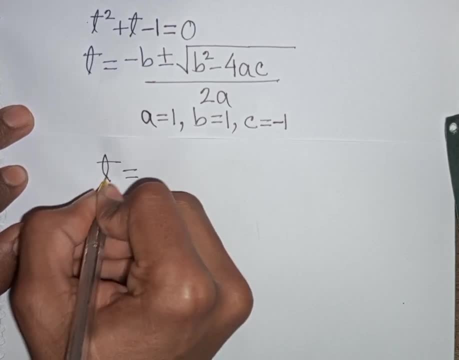 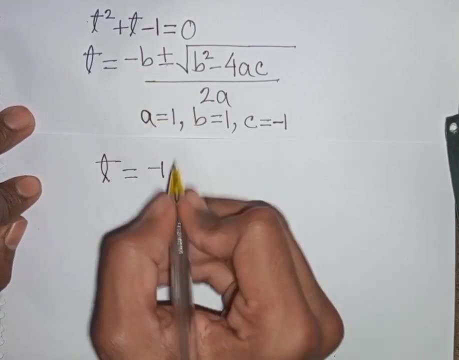 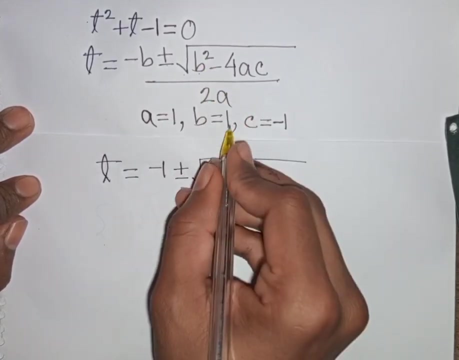 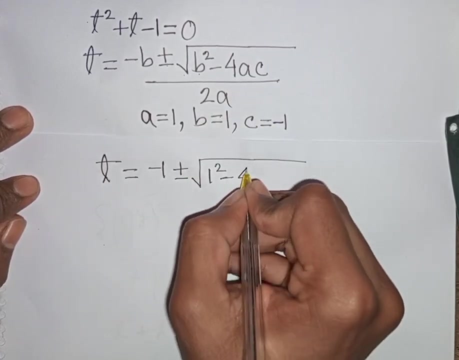 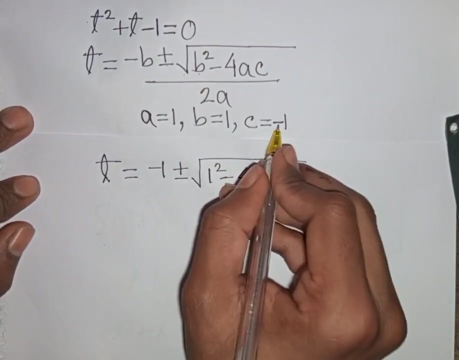 will be equal to minus b. that means 1.. Then plus or minus a square root of b square. that means it will be 1 square minus 4 times a. that means 1 times c. that means negative 1.. So bracket negative 1, then divided by: 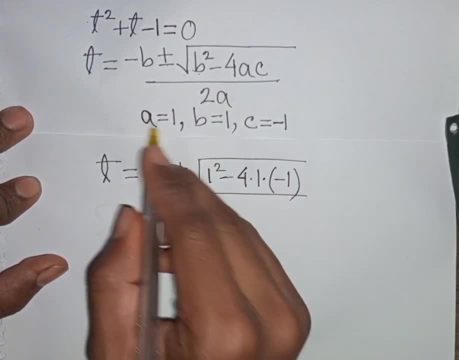 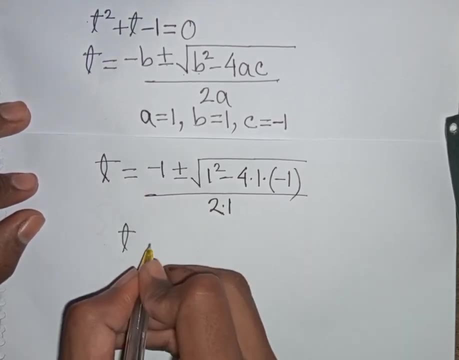 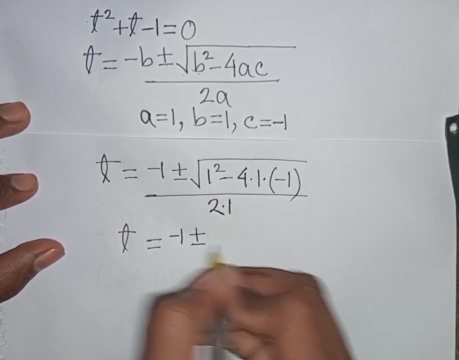 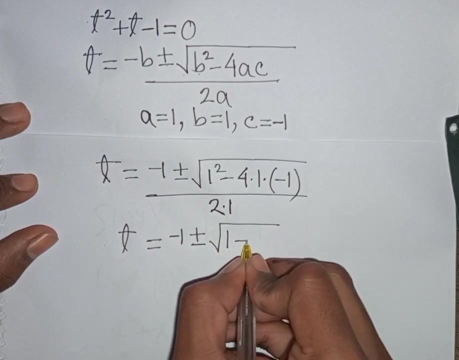 a times a, that means 1.. Now I can write here: t is equal to minus 1, plus or minus. a square root of 1 square is same as 1, then minus times minus, that means it will be plus. then 4 times 1 times 1,, that means it will be 4.. 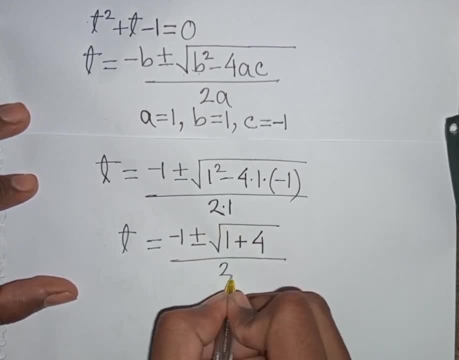 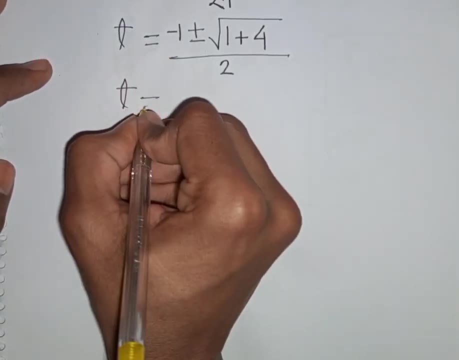 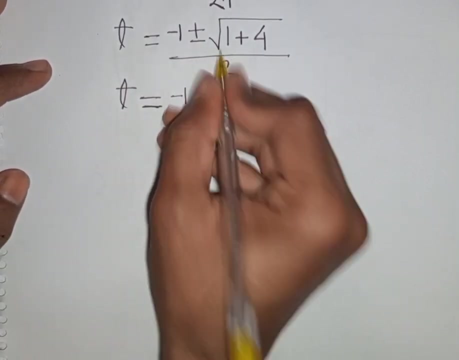 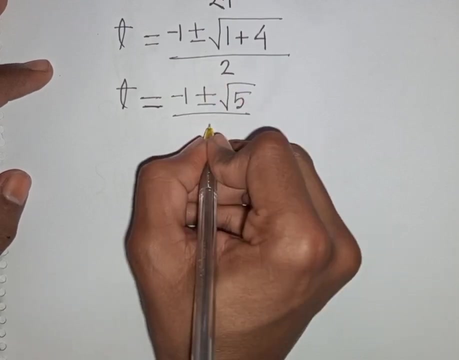 Then divided by 2 times 1, that means 2.. Now I can write here: t is equal to minus 1, plus or minus a square root of 1 plus 4, that means it will be 5, then divided by 2.. 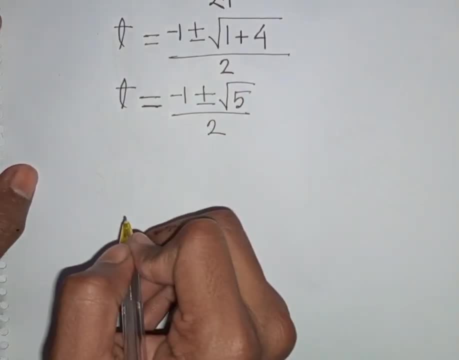 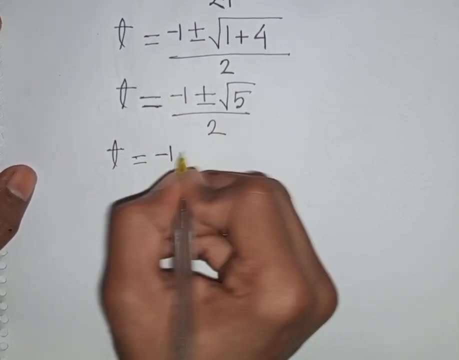 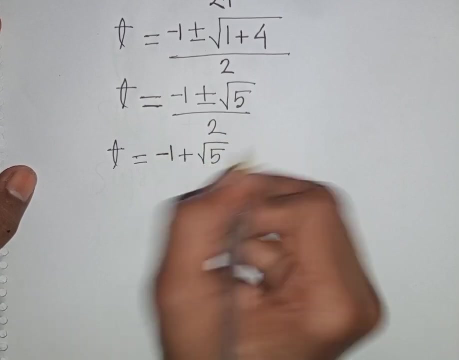 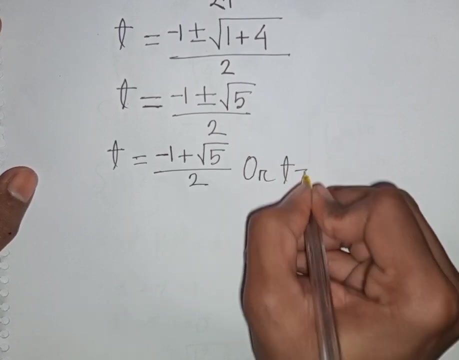 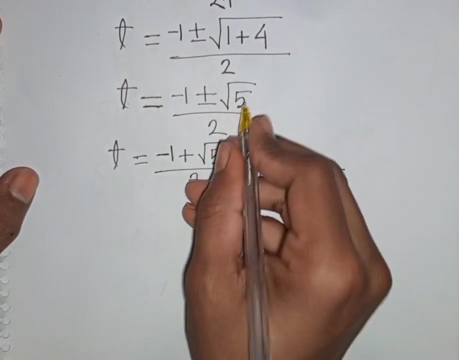 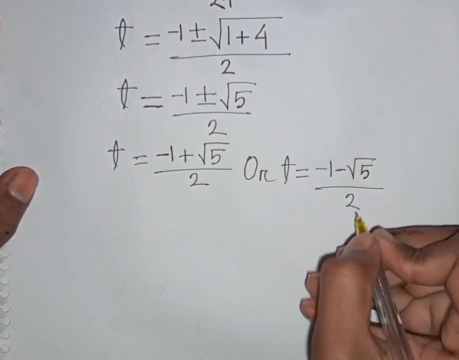 Now we see here 2 cases. So you can write here: is equal to minus 1 plus square root of 5 divided by 2, or t is equal to minus 1 minus square root of 5 divided by 2.. Now remember that let 1 by 4 bracket power x is substituted. 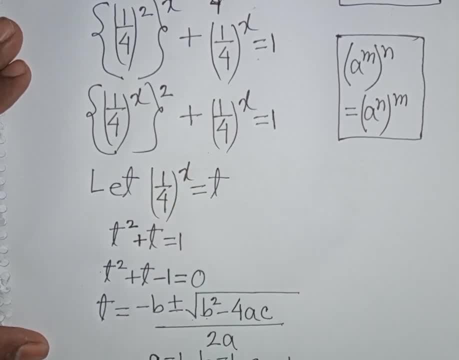 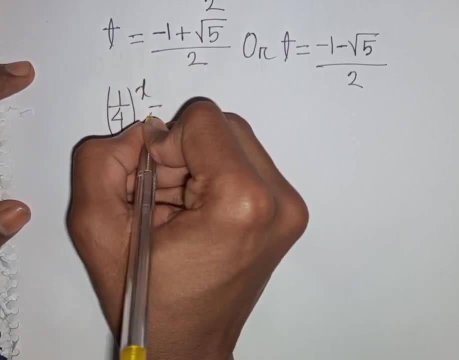 by t, So t that means 1 by 4. bracket power x, So t that means it will be 1 by 4. bracket power x is equal to plus square root of 5, that means square root of 5 divided by 2.. 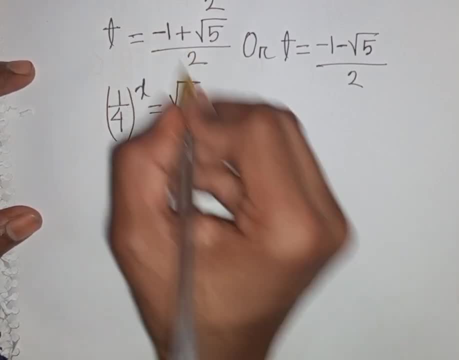 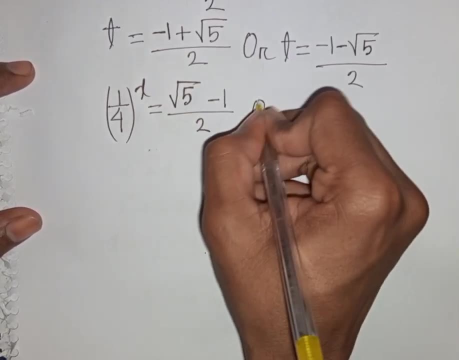 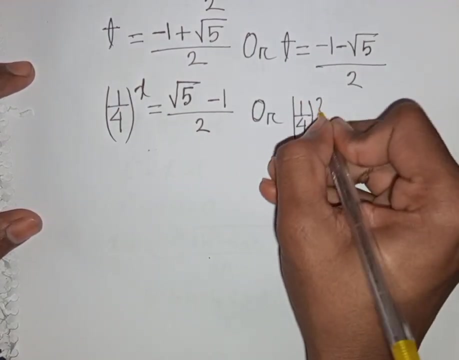 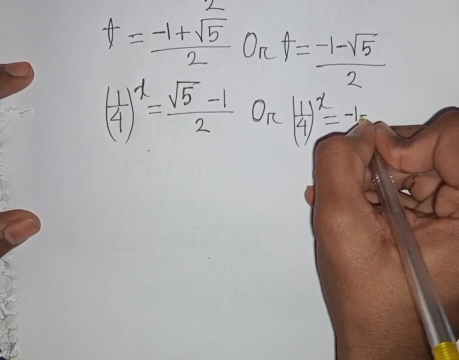 So square root of 5. then minus 1 divided by 2 or t, that means 1 by 4 bracket power x. So 1 by 4 bracket power x is equal to minus 1, minus square root of 5 divided by. 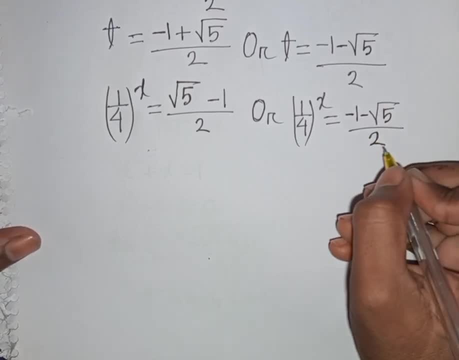 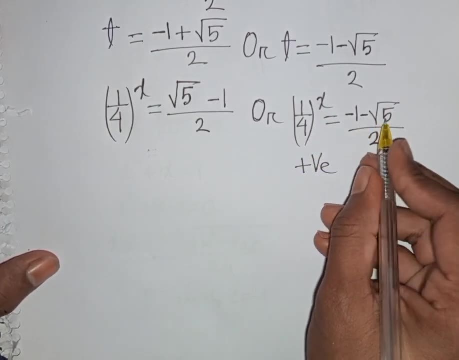 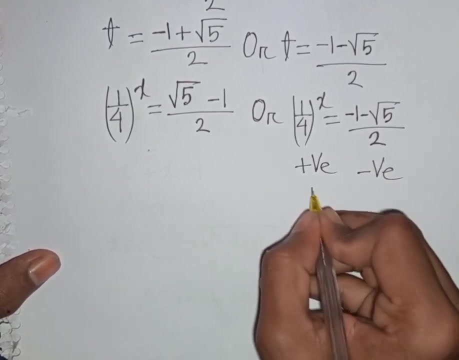 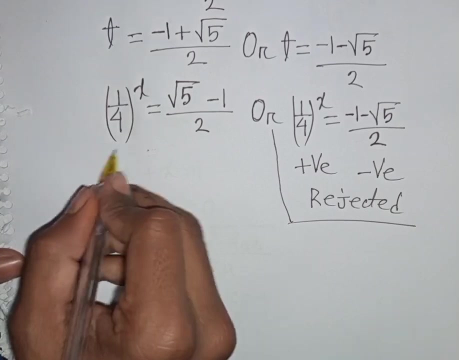 2. Now we see 1 by 4, bracket power. any number is always positive, but minus 1, minus square root of 5 divided by 2, this is must be negative. So positive cannot be equal to negative. So this is rejected. Now, from here I take log in both sides So you can write here. 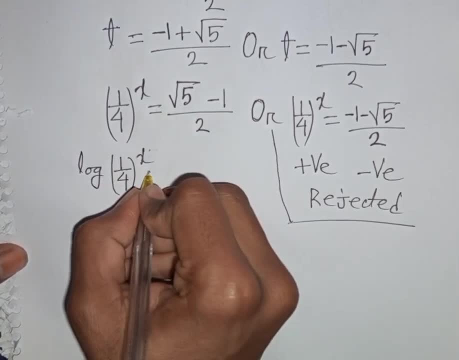 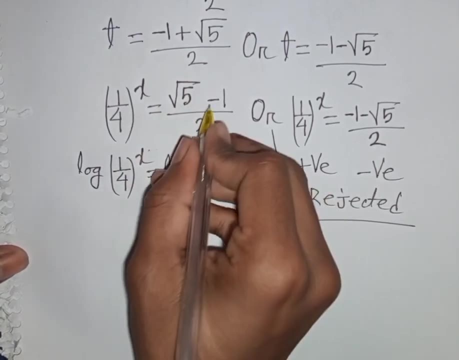 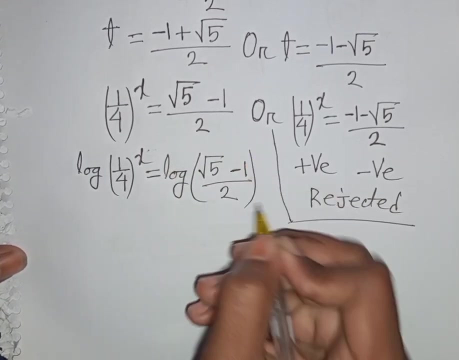 in sans wreck I can write without. So this is rejected. because for 1 by 4 bracket power x, x is equal to 1 by 4 bracket power x is equal to in. because there is no Planck equation here. log of square root of 5 minus 1 divided by 2.. Now here you can apply rule that log. 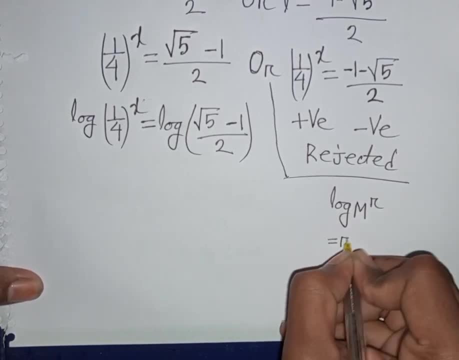 n power R is equal to R log 13.5 to 0 into 2 pi square root x by 3.. So that was своей derivative of the previous angle. Now I write my problem. When I calibrate this, I inconveniently consider pipes as cases. 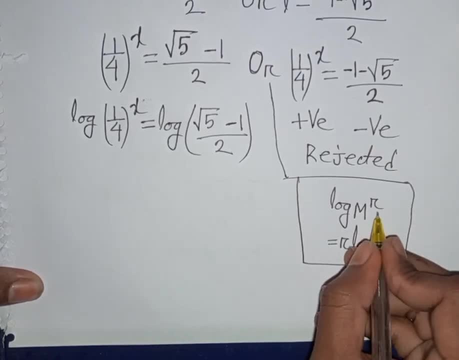 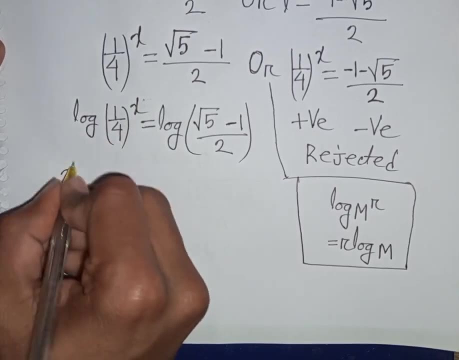 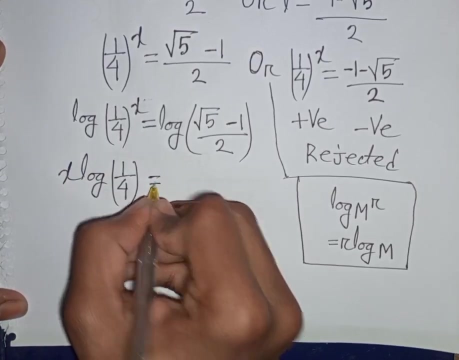 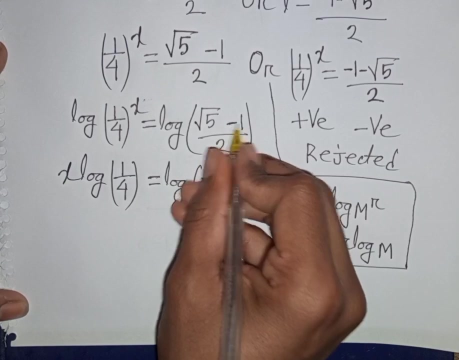 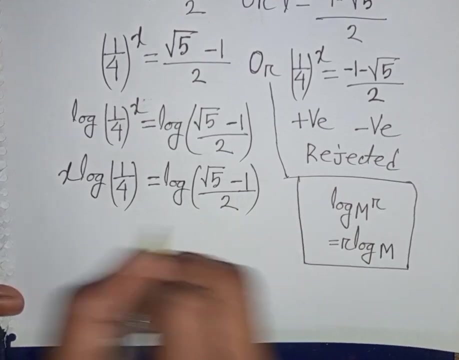 m. That means this power r move to the base. According to this rule we can compare here- This power x will move to the base. So you can write here: x log 1 by 4 is equal to log of square root of 5 minus 1 divided by 2.. Now we need the value of x, So we divide. 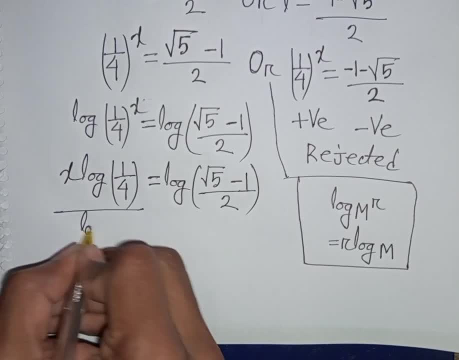 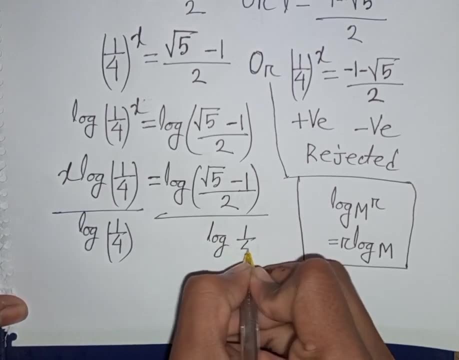 it by log of 1 by 4 in both sides. So divide it by log of 1 by 4, divided by log of 1 by 4.. Now we see this log of 1 by 4, this log of. 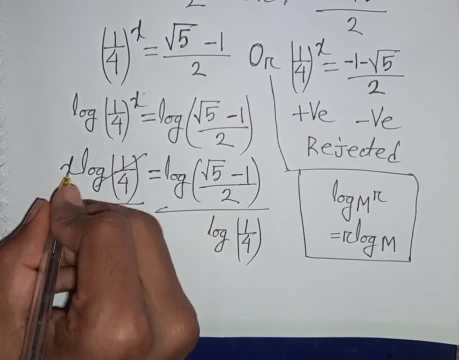 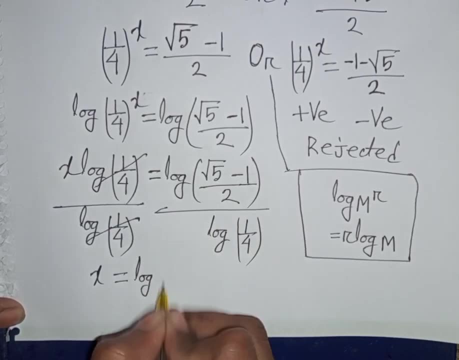 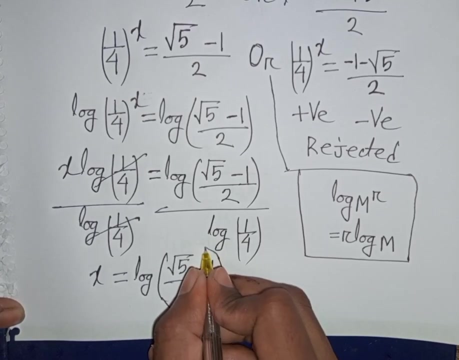 1 by 4.. This log of 1 by 4 will be cancelled. So here x will be equal to this. divided by this, That means it will be log of square root of 5 minus 1 over 2, then base of 1 by 4.. So. 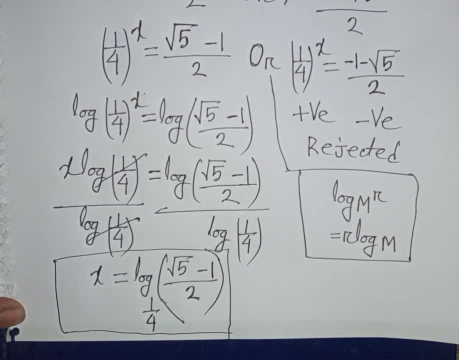 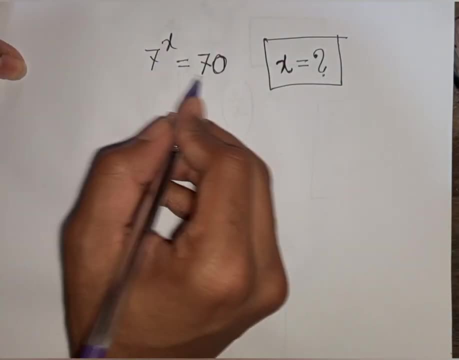 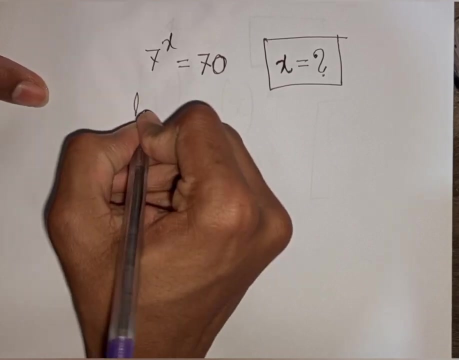 this is the value of x. So this is our final How to solve 7 power x is equal to 70?. Find the value of x. So at first we take log in both sides So you can write here log. 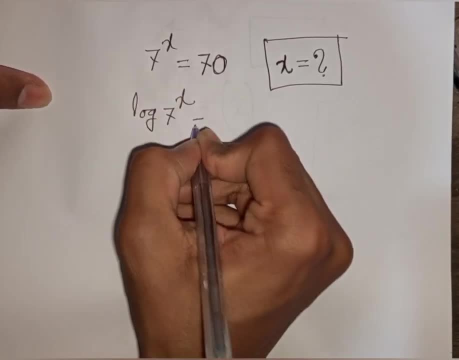 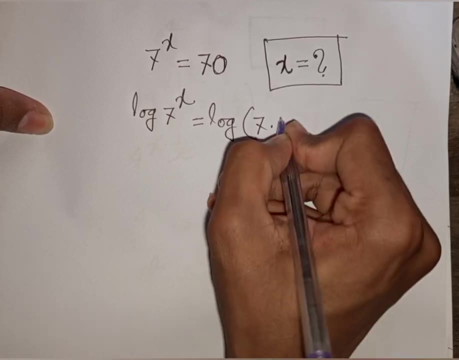 of 7, power x is equal to log of 70- can be written as 7 times 7.. So this is the value of x. So this is the value of x. So this is the value of x. So this is the value of.